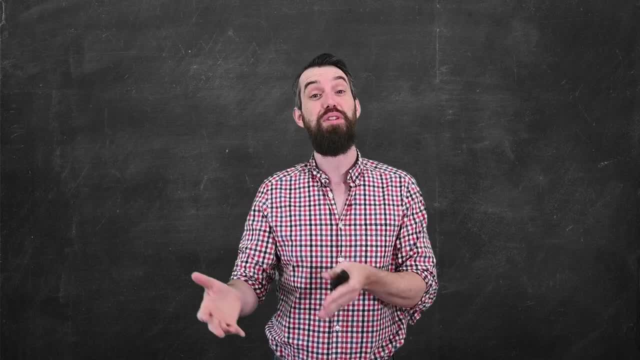 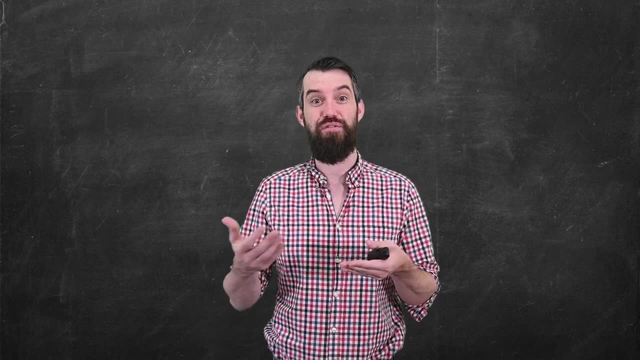 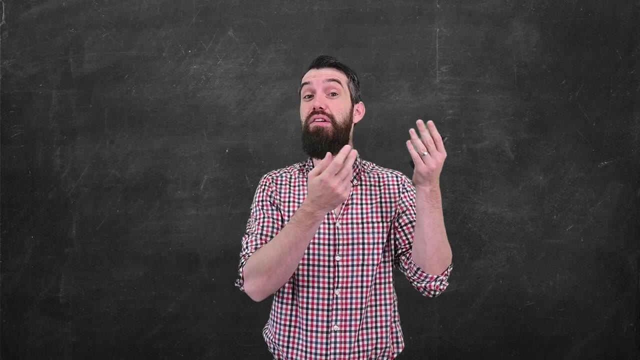 How should we define differentiability of a multivariable function? Well, if you've seen the previous video in this Calculus 3 playlist, the video on partial derivatives, you might think that we've already got an answer. Partial derivatives are the higher dimensional analog of the derivative back in single variable. 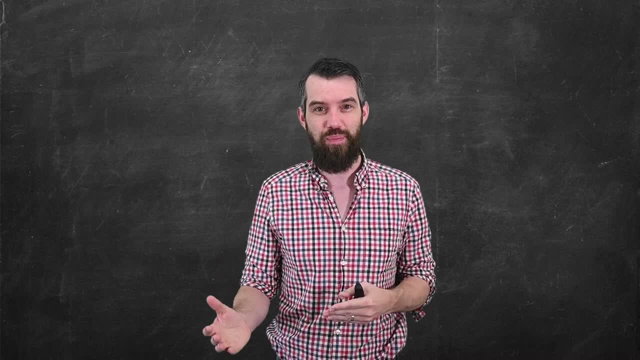 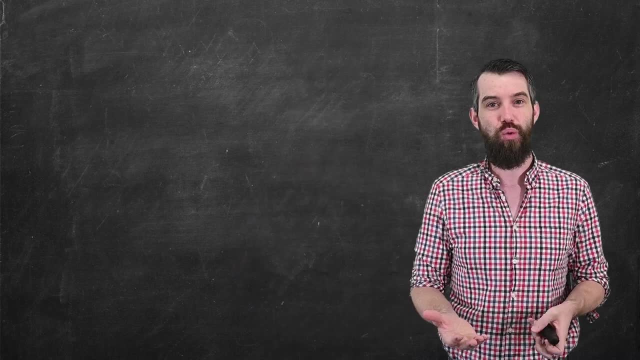 calculus, But unfortunately it's not quite so simple And in this video I really want to explore why- Why we need something more than partial derivatives. So we're going to see an example where we're going to talk about continuity, And continuity is a very important property that a 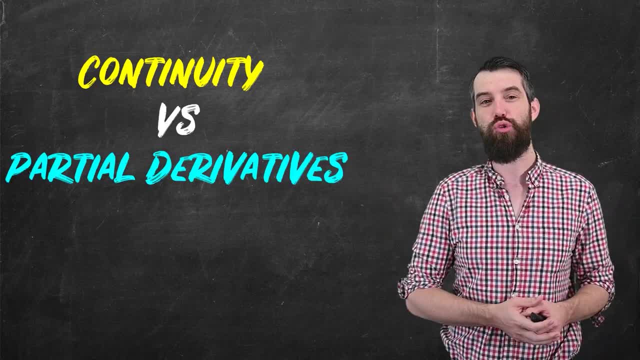 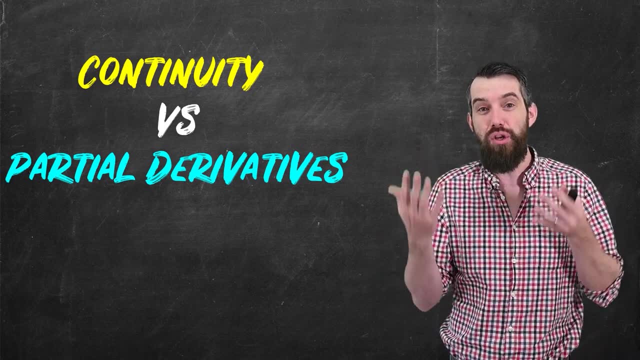 function can have. We're going to talk about whether they have partial derivatives and what the relationship between continuity and partial derivatives is, And then we're going to see that we're actually going to need an entirely new concept, one that we're going to call. 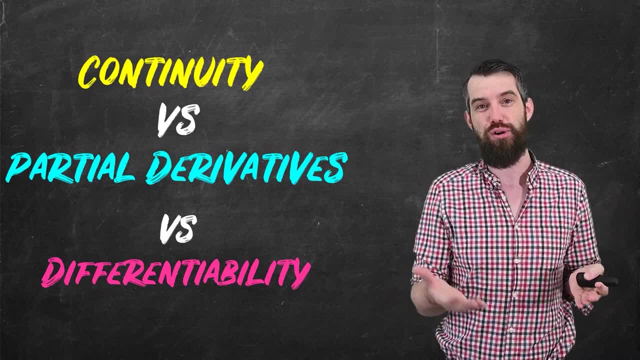 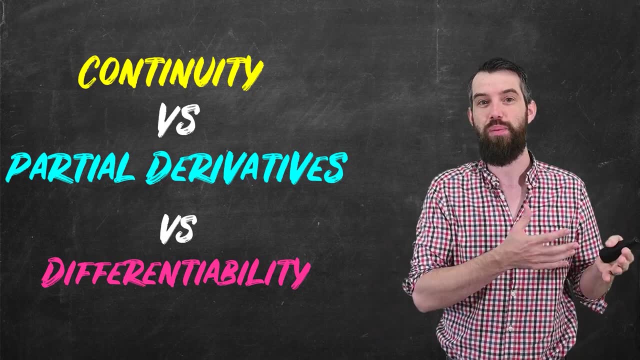 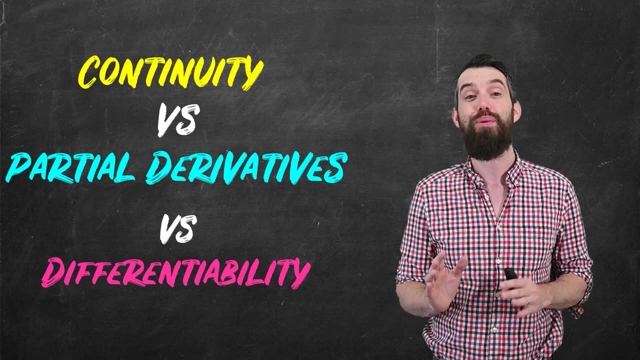 differentiability that is separate from just having partial derivatives, And so that final answer about differentiability we're actually going to need is a concept called differential to introduce in the next video in this multivariable calculus series. Now, before we dive into the multivariable situation, let me just briefly remind you of what 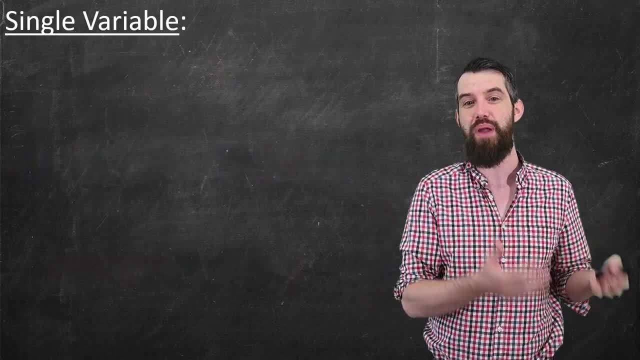 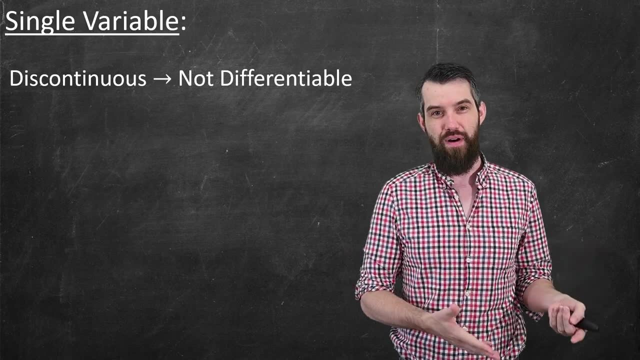 was going on in single variable calculus, so that we have something to compare to Now. in single variable calculus there was a very important relationship. If you had a discontinuity of a function, then the function was not differentiable. And then the counterpositive of that statement is that 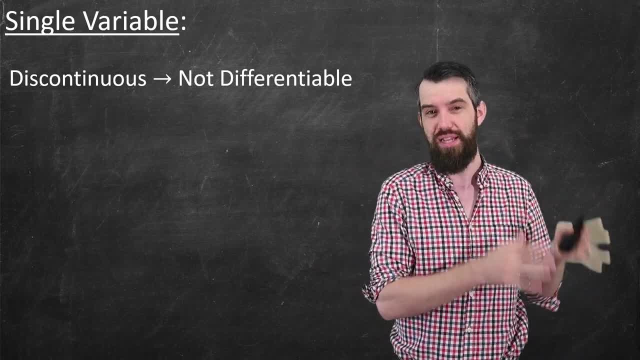 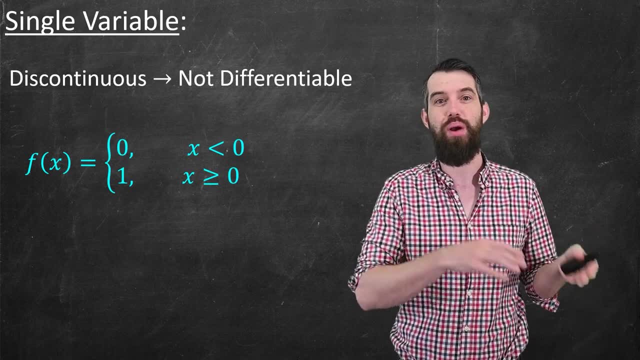 if you have a differentiable function, it had to be continuous. An example that kind of illustrates this point is well, a step function, The function that's 0 when x is less than zero and 1 when x is greater than or equal to zero. It just 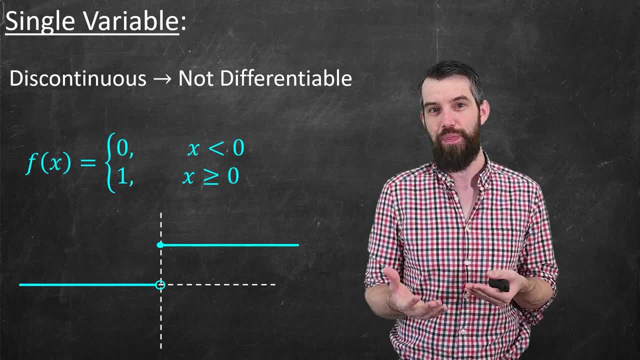 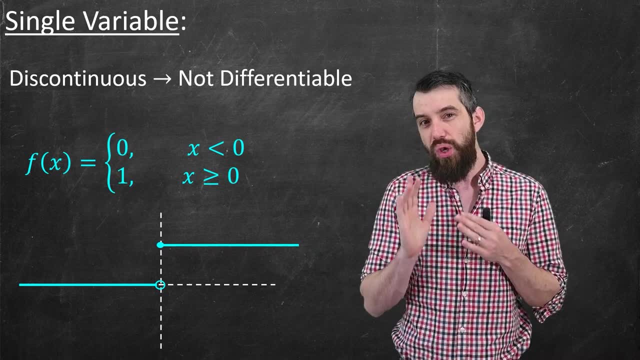 looks like this. It looks like a little step. Now it's clearly not continuous. at the point x equal to zero there's this jump at x equal to zero, But nor is it differentiable at x equal to zero If you think about what the derivative 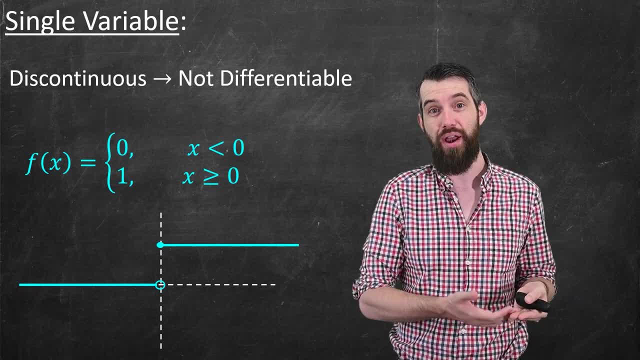 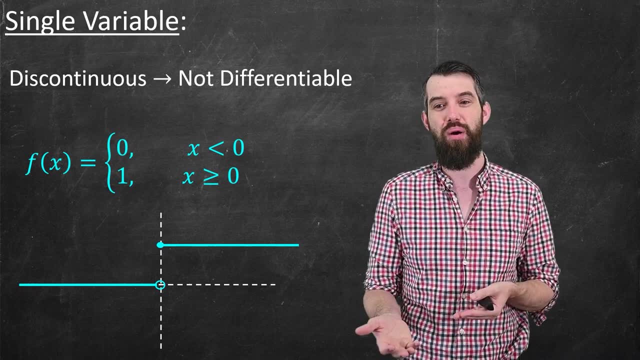 did. it was trying to be sort of a differential function, but it was also trying to be to put a tangent line on at some particular point. But how could you ever put a tangent line to the curve at the value of x equal to zero? And so this: 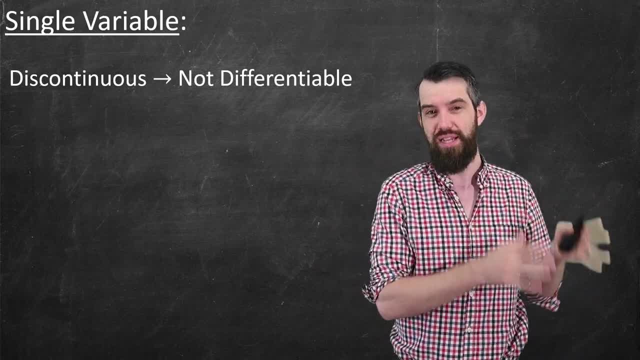 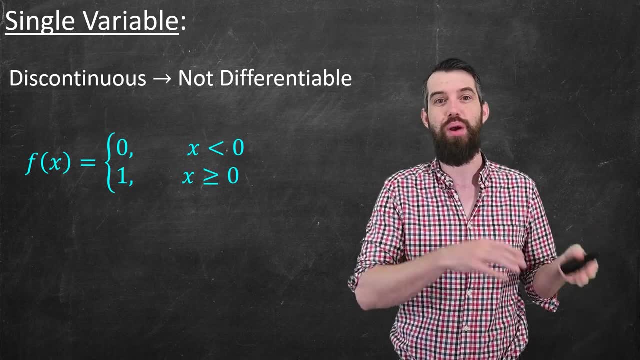 if you have a differentiable function, it had to be continuous. An example that kind of illustrates this point is well, the step function, The function that's zero when x is less than zero and one when x is greater than or equal to zero. 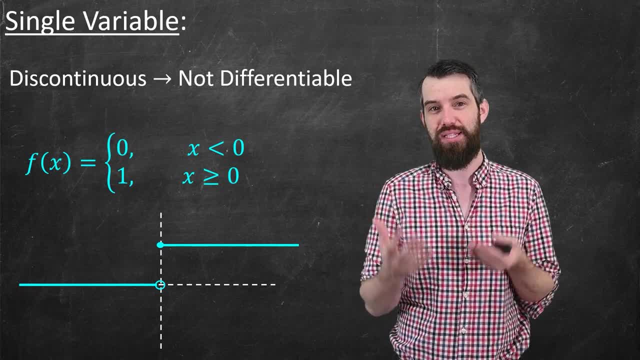 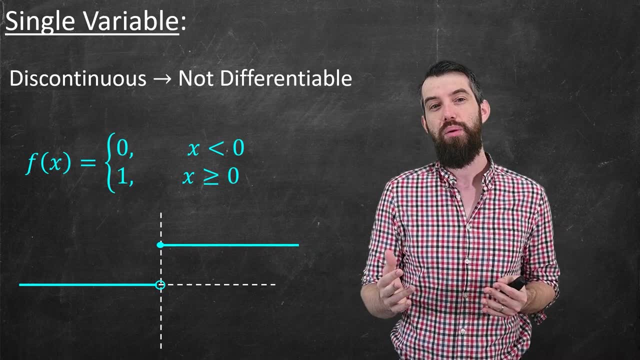 This just looks like this. It looks like a little step. Now it's clearly not continuous. at the point x equal to zero, There's this jump at x equal to zero, But nor is it differentiable at x equal to zero If you think about what the 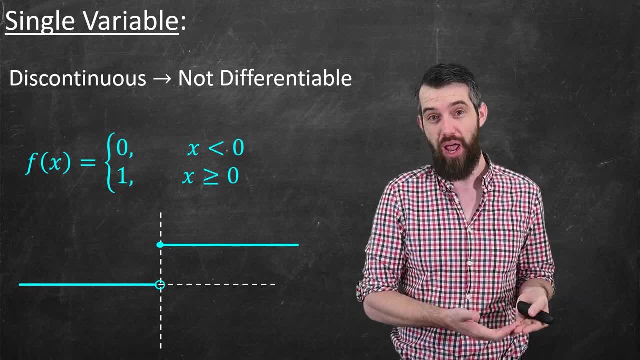 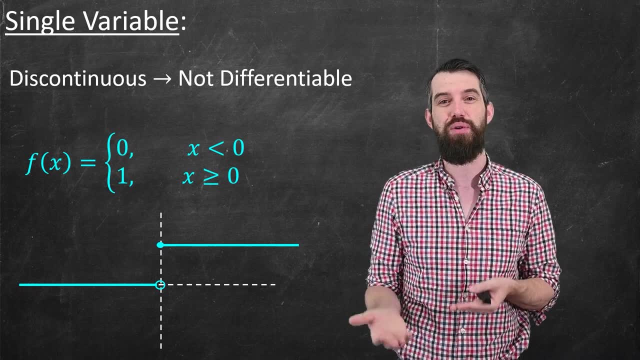 derivative did. it was trying to to put a tangent line on at some particular point. But how could you ever put a tangent line to the curve at the value of x equal to zero? And so this example was one such example where it was neither continuous nor differentiable. 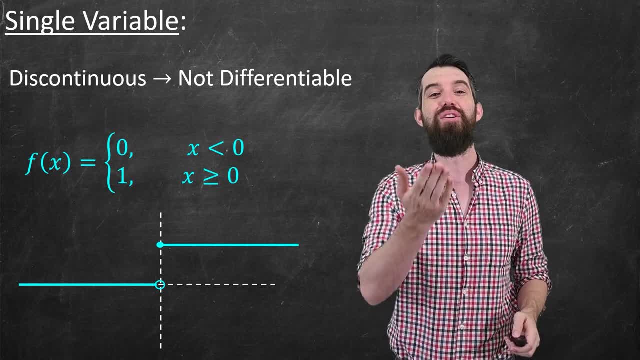 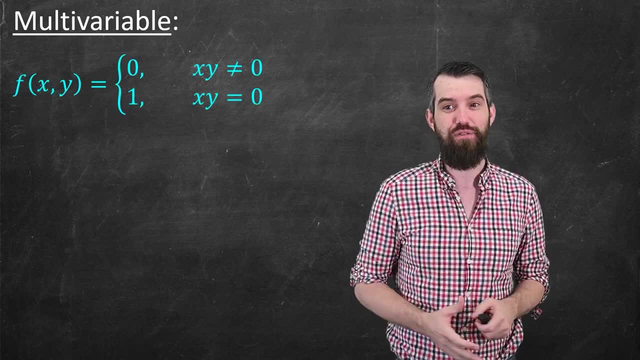 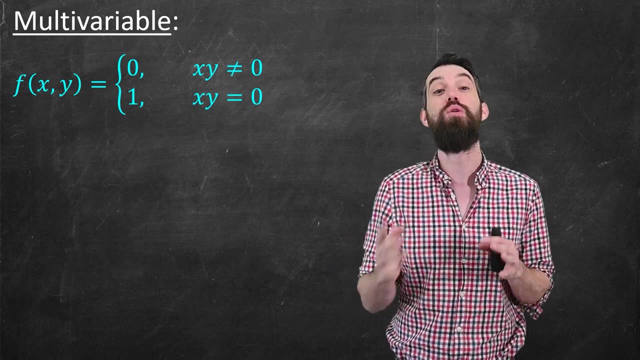 But look what happens in sort of the higher dimensional analog of this exact same function. So we're talking about multivariable calculus now, and the function we're going to talk about looks superficially very similar. It's zero for x- y not being equal to zero, and then one for x- y equaling zero, x- y equaling zero. 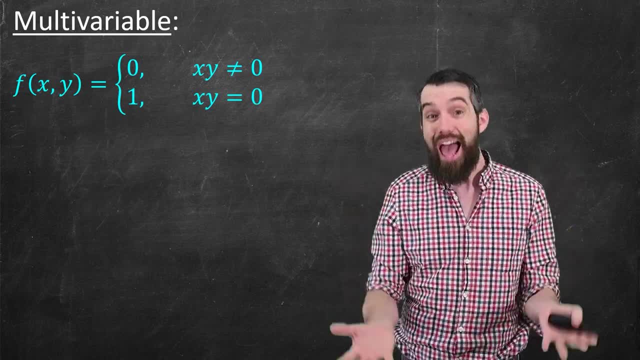 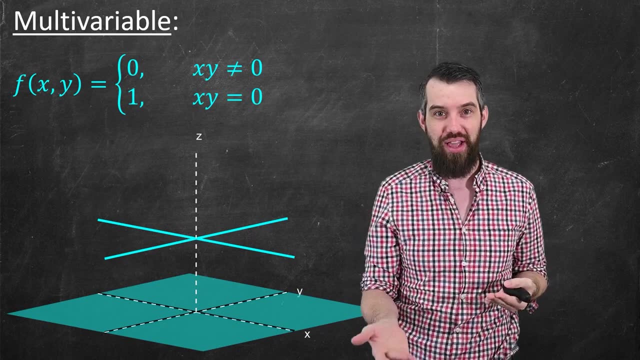 is just saying either x is zero or y is zero. Those are the axes, and so this is what it actually looks like. It looks like a cross Above the axes. where x is zero or y is equal to zero, the function has a height: 1. Everywhere else, it has a. 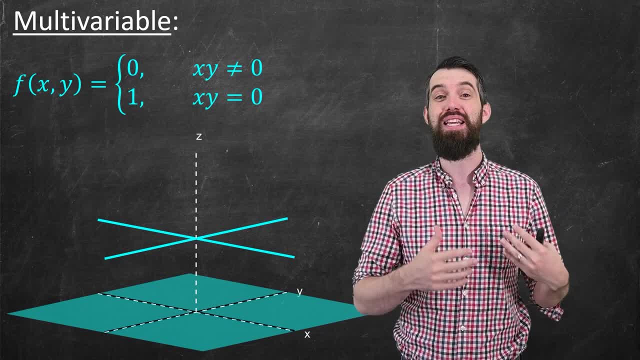 height 0.. Now, I really love this function because, as we're going to see, it helps to illustrate some of the core ideas of multivariable calculus. So let's try to answer the same questions. So let's try to answer the same questions. 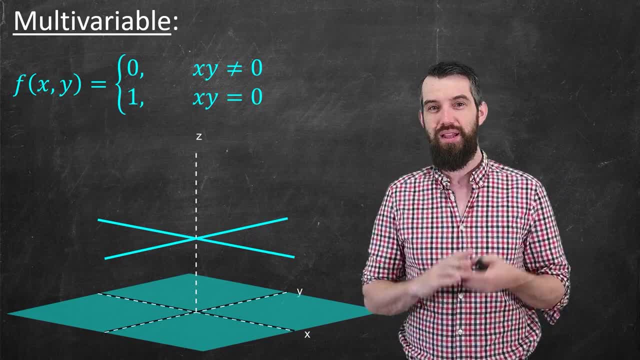 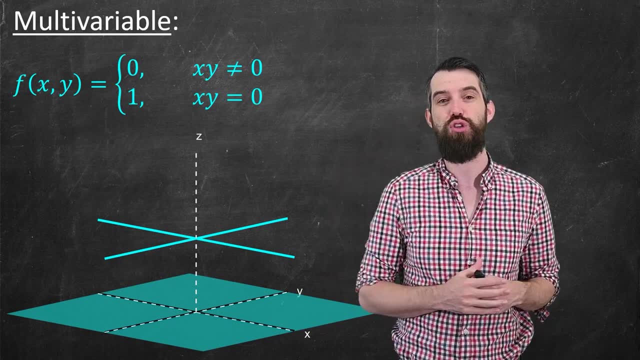 So let's try to answer the same questions. Is this function continuous and does it have partial derivatives? Now, just looking at the function makes it appear that it's not continuous. Indeed, it's going from zero and then it jumps right up to one, and that kind of jump, we think. 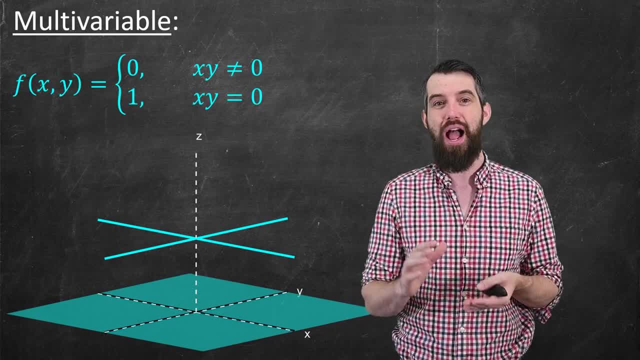 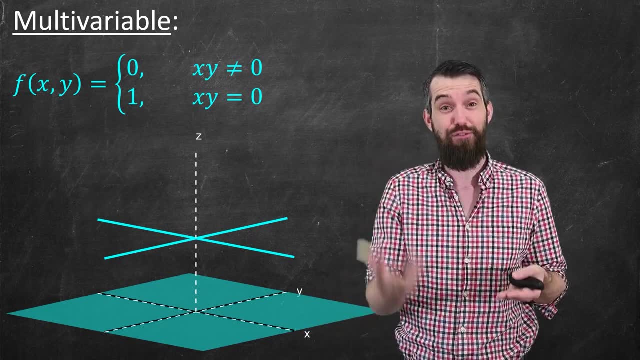 of as something being not continuous, But perhaps we should try to actually state that a little bit more precisely with limits. because what is continuity? It means that the limit exists and the function exists and they are equal. So let's compute the limits of this particular thing. I want to take first 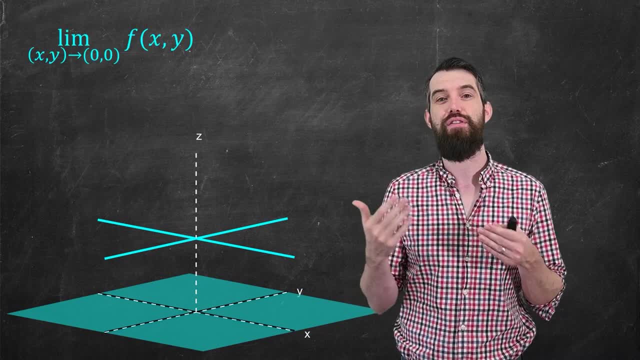 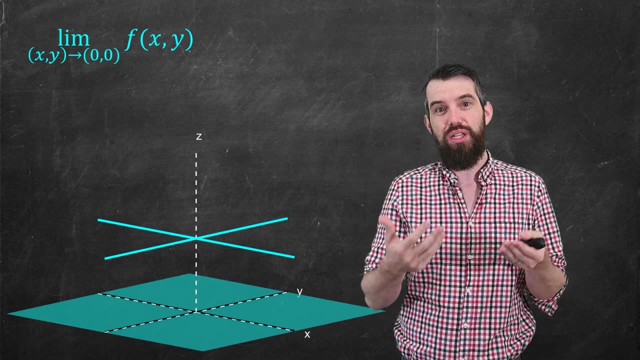 the limit going to 0, 0 of this function f of x, y. Now, when we first introduced limits in this multivariable calculus course, we saw that we could do limits along a bunch of different paths, And so I'm going to first begin with a path which is going along y equal. 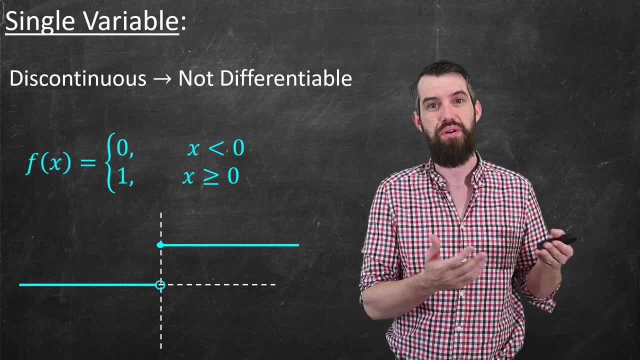 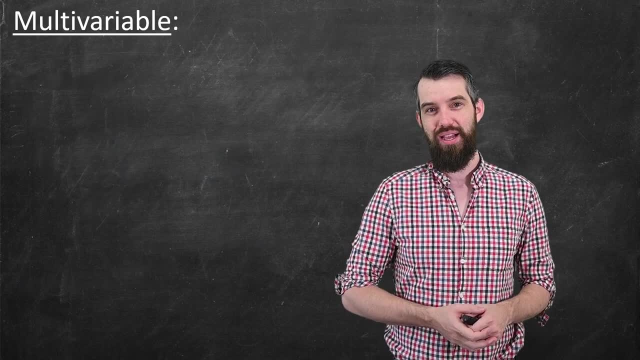 example was one such example, where it was neither continuous nor differentiable. But look what happens in sort of the higher dimensional analog of this exact same function. So we're talking about multivariable calculus now, and the function we're going to talk about looks superficially very similar: It's zero, for 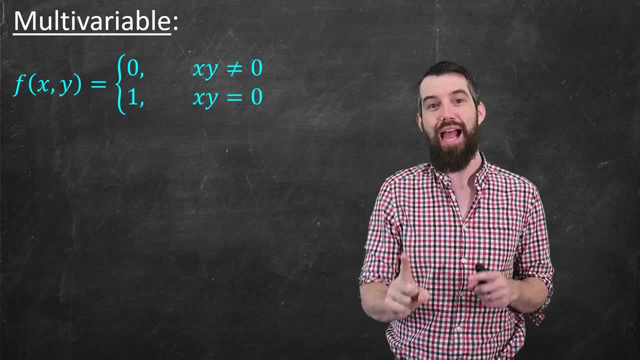 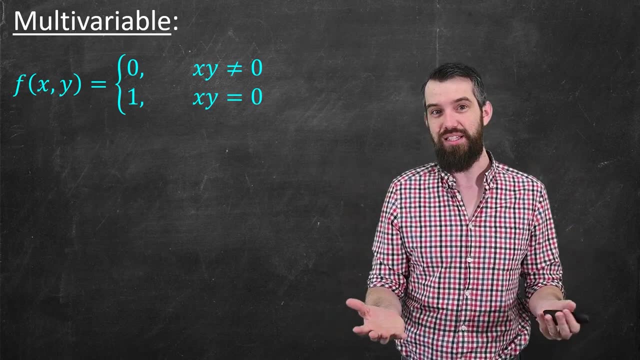 x- y not being equal to zero, and then one for x- y equaling zero. x- y equaling zero is just saying either x is zero or y is zero. Those are the axes, and so this is what it actually looks like. It looks like a cross Above the axes where x is. 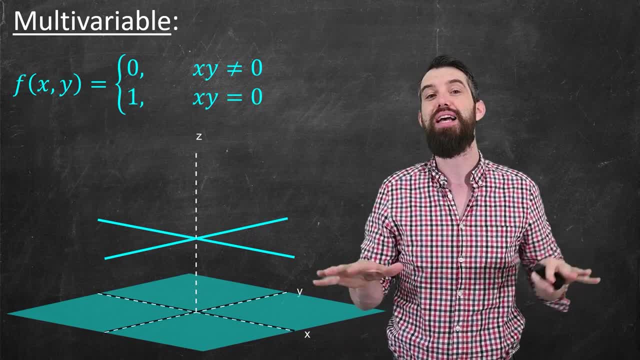 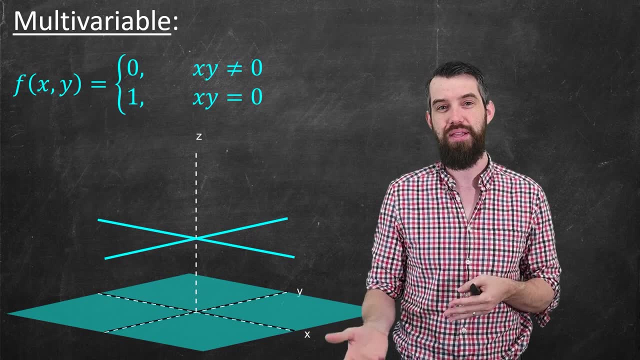 zero or y is equal to zero, the function has a height 1.. Everywhere else it has a height 0.. Now I really love this function because, as we're going to see, it helps to illustrate some of the core ideas of multivariable calculus. So let's try to. 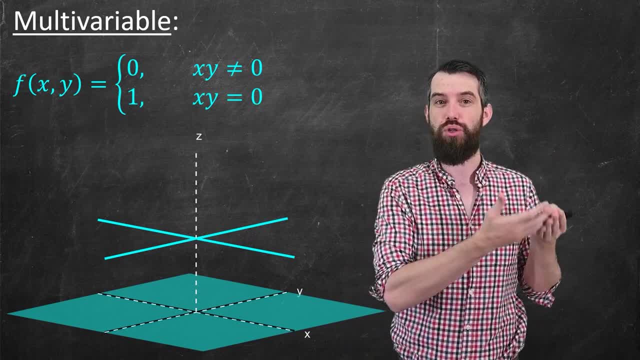 answer the same questions. So let's try to answer the same questions. So let's try to answer the same questions. Is this function continuous and does it have partial derivatives? Now, just looking at the function makes it appear that it's not continuous. Indeed, it's. 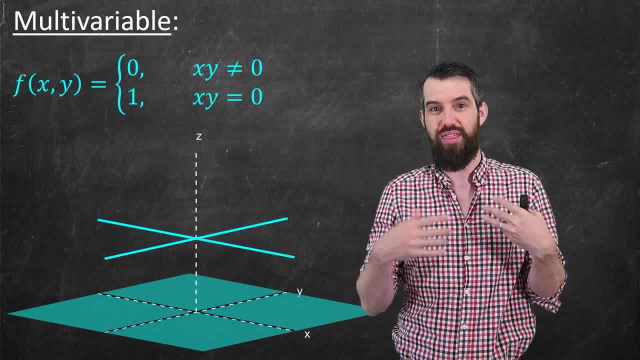 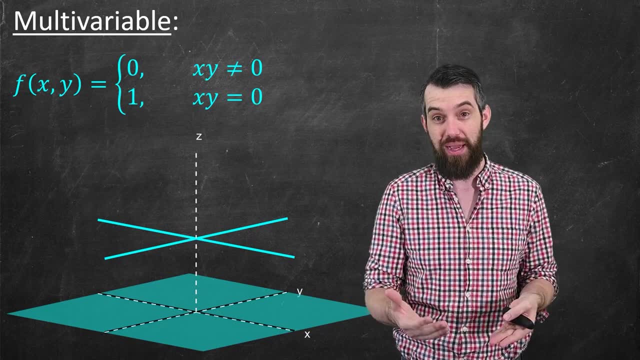 going from zero and then it jumps right up to one, and that kind of jump we think of as something being not continuous. But perhaps we should try to actually state that a little bit more precisely with limits, because what is continuity? It means that the limit exists and the function exists and they are equal. So 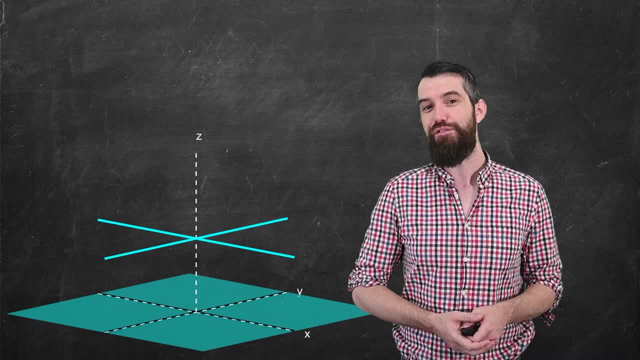 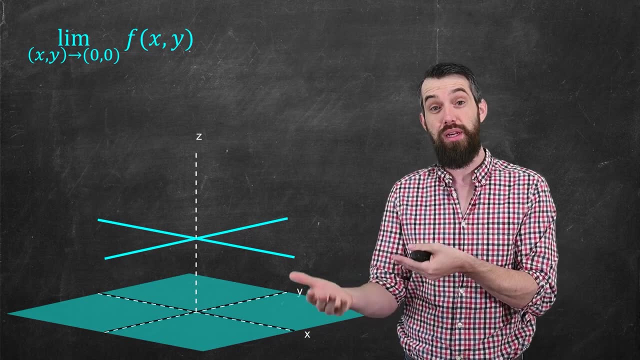 let's compute the limits of this particular thing. I want to take first the limit going to 0, 0 of this function f of x, y. Now, when we first introduced limits in this multivariable calculus course, we saw that we could do limits along a bunch. 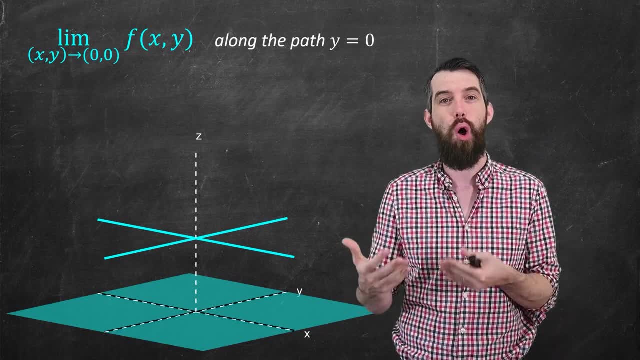 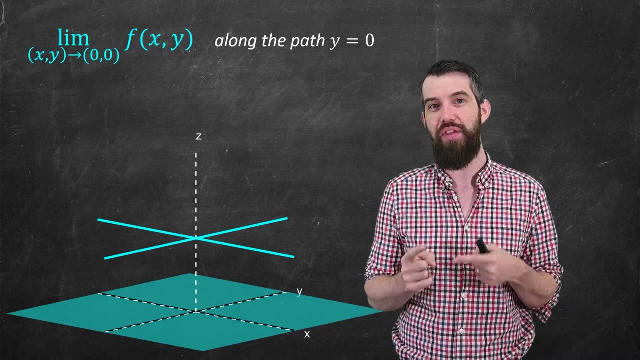 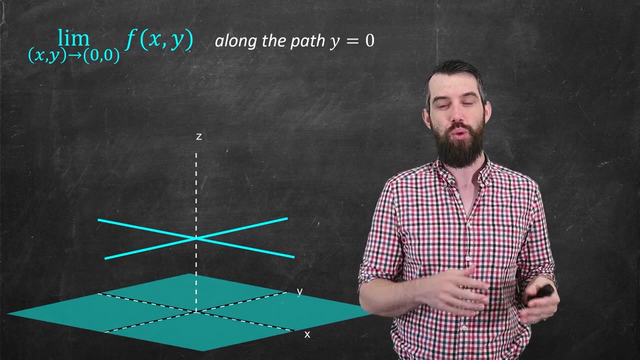 of different paths, And so I'm going to first begin with a path which is going along y equal to zero, In other words, this is just the x-axis. Now, along this path, if you're going along the x-axis, well, that function is 1 everywhere where y is zero. So, according to this path, 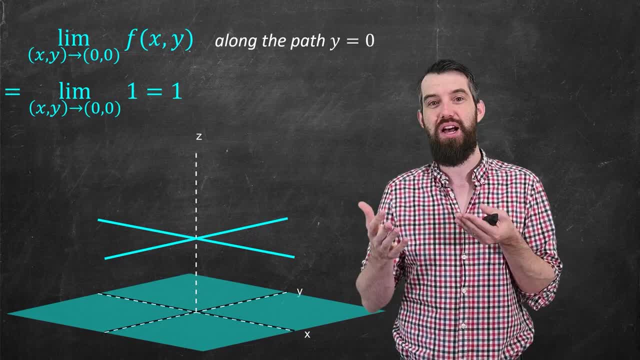 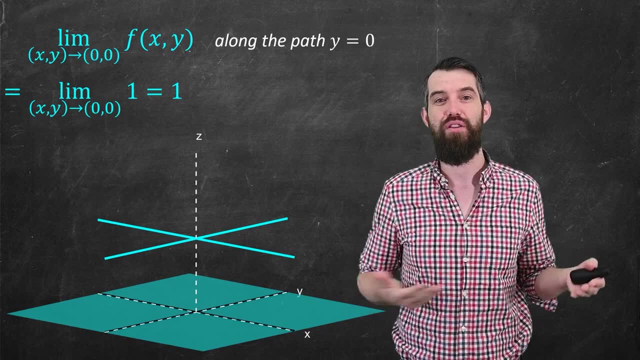 this is just taking the limit of the function 1, and of course the limit of the function 1 is just well 1.. So the point is that this path does not see the anywhere where the function is zero. It only sees. 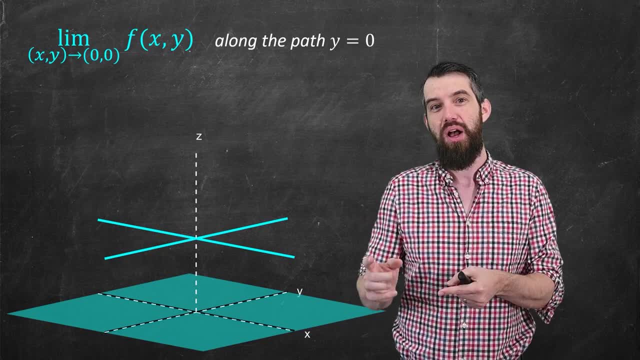 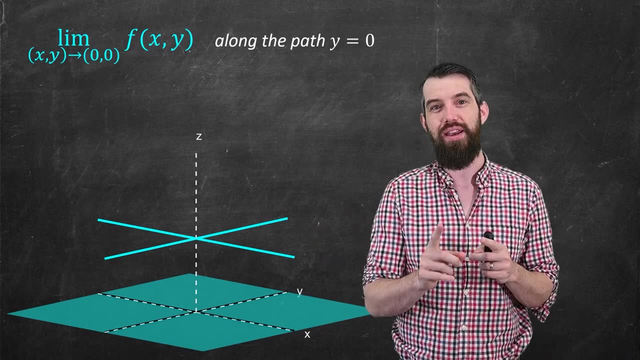 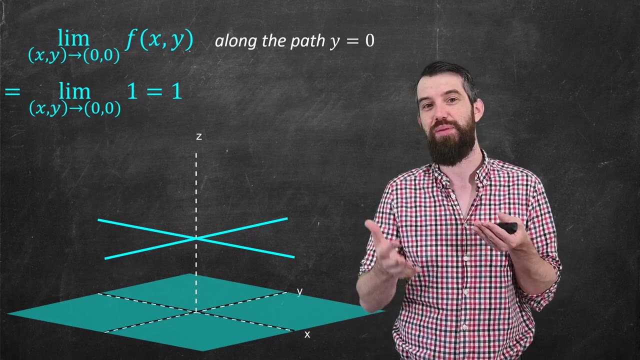 to zero. In other words, this is just the x-axis. Now, along this path, if you're going along the x-axis, well, that function is 1 everywhere where y is zero. So, according to this path, this is just taking the limit of the function 1, and, of course, the limit of the function 1 is just, well, 1.. 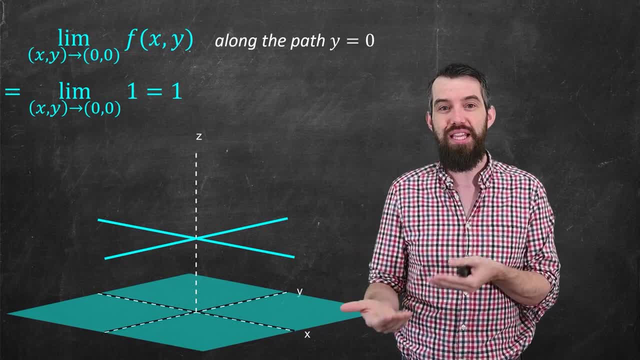 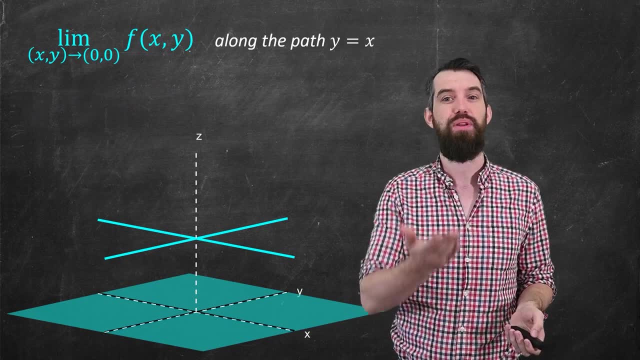 So the point is that this path does not see anywhere where the function is zero. It only sees where the function is 1.. And so it appears that the limit is 1.. Okay, let me do a different path, though. Now I'm going to take the path which has changed to be y equal to x instead. 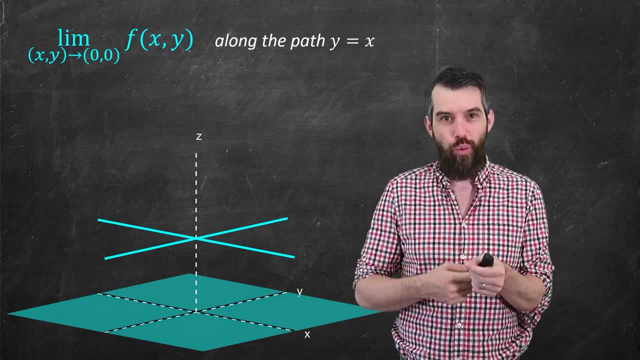 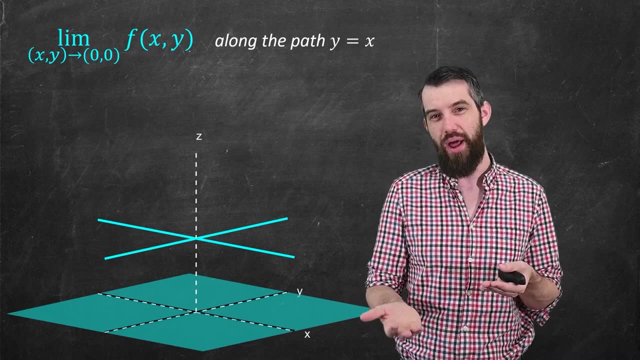 So these are numbers like 1, 1,, half half, 0.1, 0.1.. But what is f of a number like 0.1, 0.1?? Well, anywhere that was not an axi, we saw that it was zero. 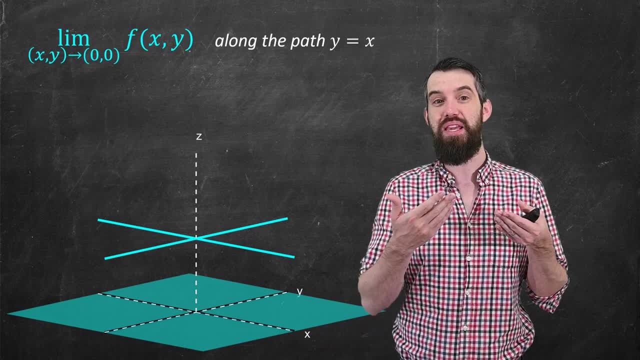 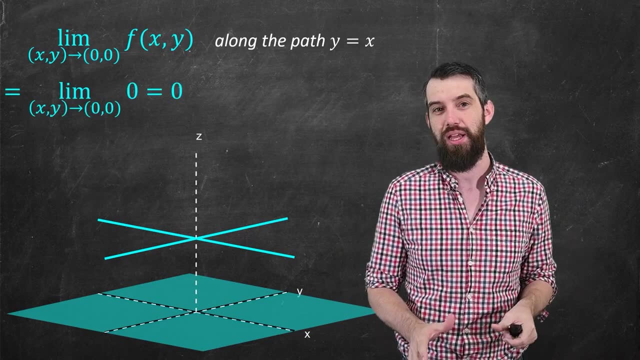 So, along this path, y equal to x, it's going to be, in fact, zero everywhere, except for this case, when x is actually equal to zero and y is actually equal to zero, which the limit doesn't care about. And so, as a result, what is this limit of? This is the limit of things that are zero and less, just zero. 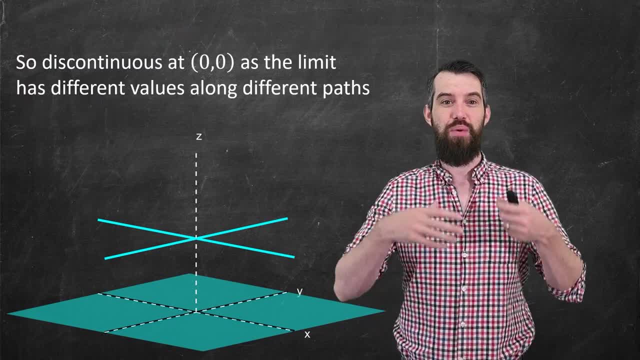 Okay. so what's the big takeaway here? Now we've seen that, indeed, we have two different paths, and the limit along the x-axis is 0.. So what's the big takeaway here? Now, we've seen that, indeed, we have two different paths. and the limit along the y-axis is 0.. So what's the big takeaway here? Now we've seen that indeed, we have two different paths and the limit along the y-axis is 0.. So what's the big takeaway here? Now, we've seen that, indeed, we have two different paths. 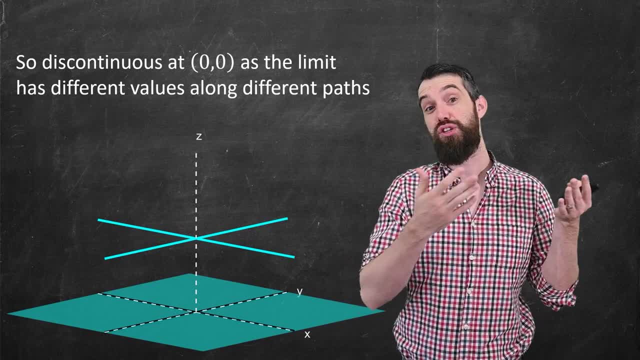 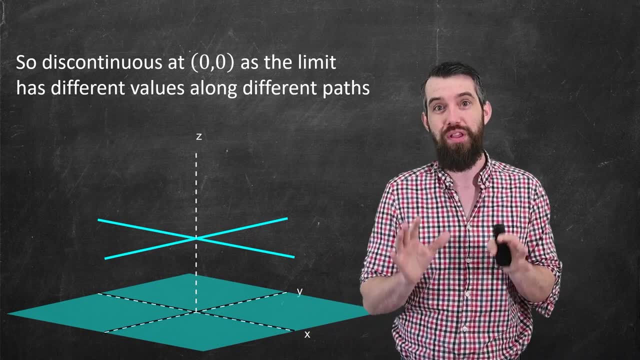 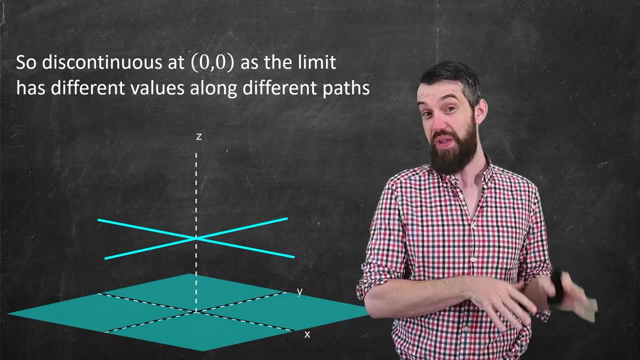 gives two different values, and so the limit does not exist. The limit does not exist, the function is not continuous, because continuity meant that the limit existed and equaled the function value. So in this case we have proven that no, it matches our intuition: It is not continuous. 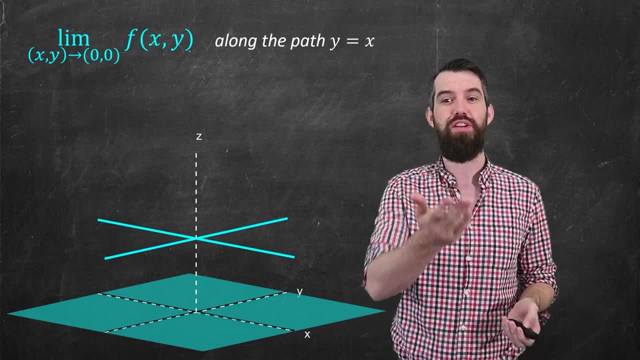 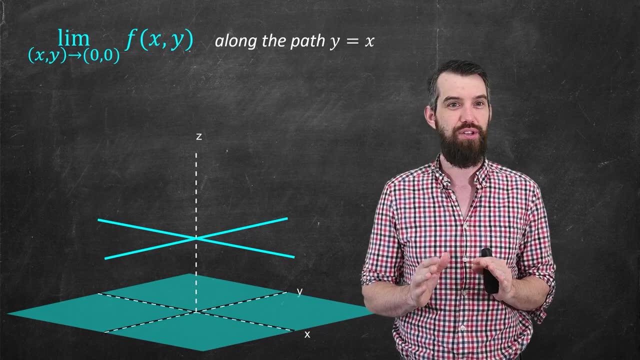 where the function is 1,, and so it appears that the limit is 1.. Okay, let me do a different path, though Now I'm going to take the path which has changed to be y equal to x instead, So these are numbers like 1, 1, half, half, 0.1, 0.1. 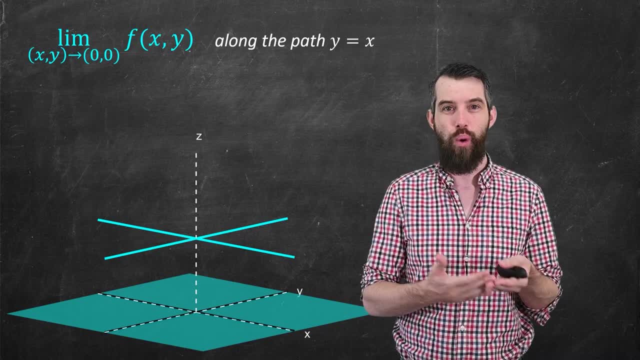 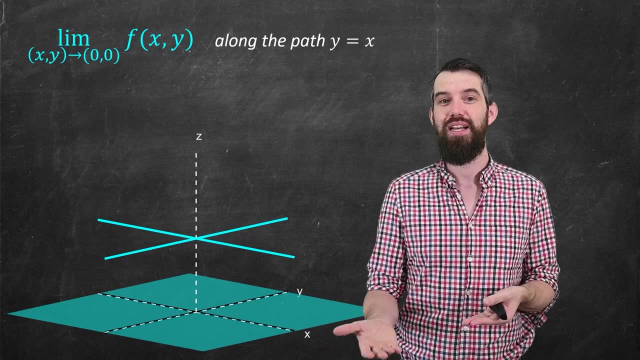 But what is f of a number like 0.1, 0.1?? Well, anywhere that was not an axi, we saw that it was zero. So, along this path, y equal to x, it's going to be, in fact, zero everywhere, except for this case. 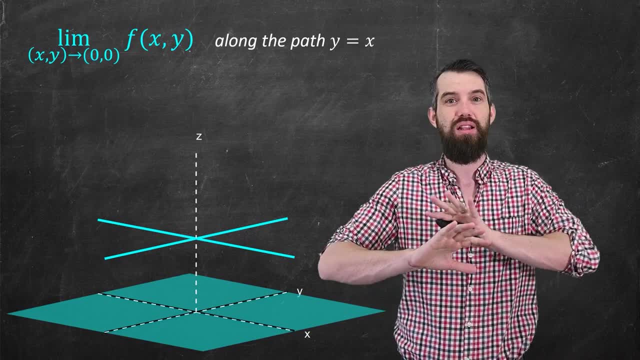 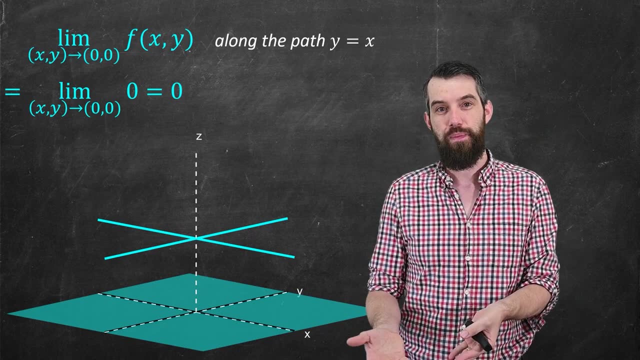 when x is actually equal to zero and y is actually equal to zero, which the limit doesn't care about. And so, as a result, what is this limit of? This is the limit of things that are zero and less, just zero. Okay, so what's the big takeaway here? Now, we've seen that, indeed, we have two different paths. 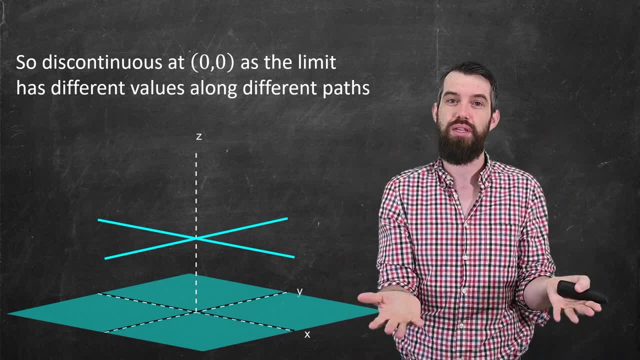 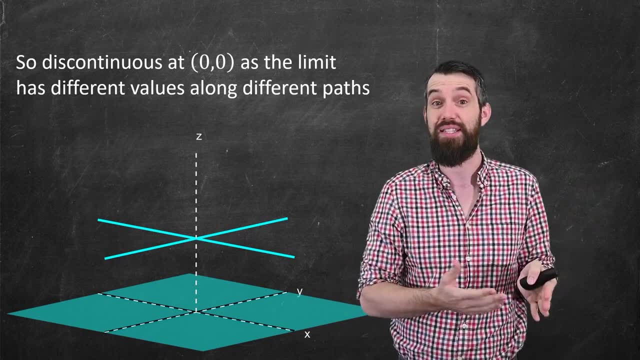 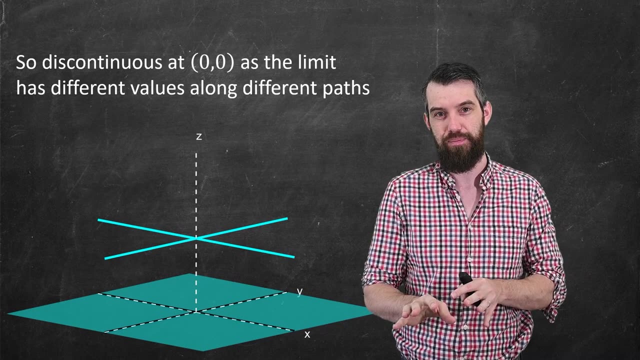 and the limit along those two different paths gives two different values, and so the limit does not exist. The limit does not exist, the function is not continuous, because continuity meant that the limit existed and equaled the function value. So in this case we have proven that no, it matches our intuition. it is not continuous. 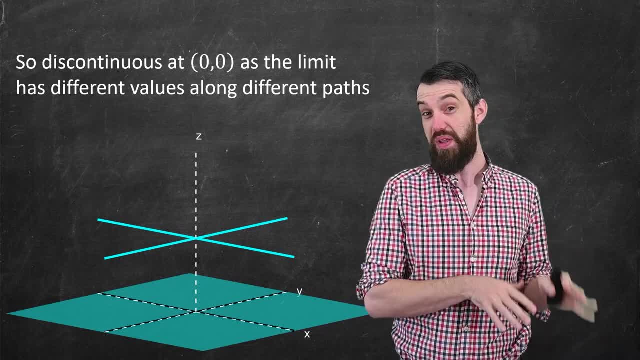 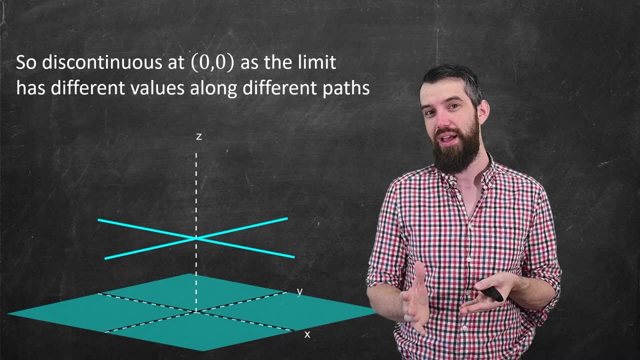 Okay. so if what was true in calculus 1 was true here, we would therefore be able to immediately say that the partial derivatives did not exist. That's what we might hope for. Unfortunately, it's not quite so simple. So let's try to study the partial derivatives and see what happens to them. 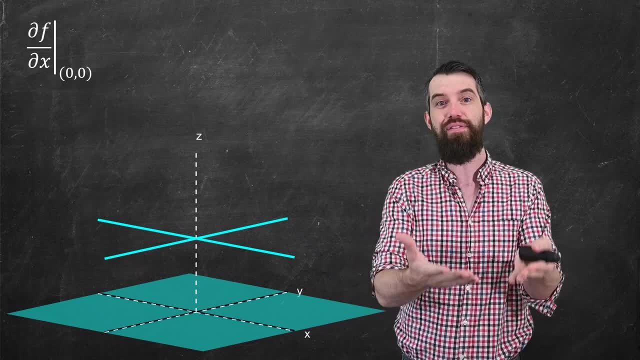 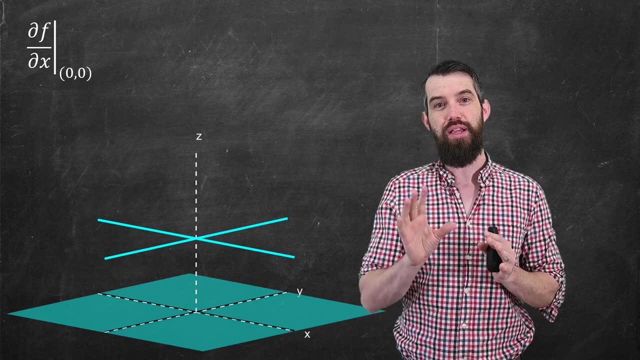 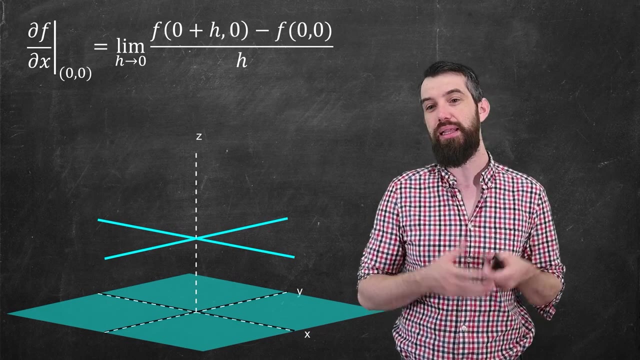 So let's do the partial derivative with respect to x first, So partial derivative of f with respect to x and at the point. So that's what the vertical bar means, evaluated at The definition of partial derivatives, as we've seen previously, is well, it's analogously a limit. 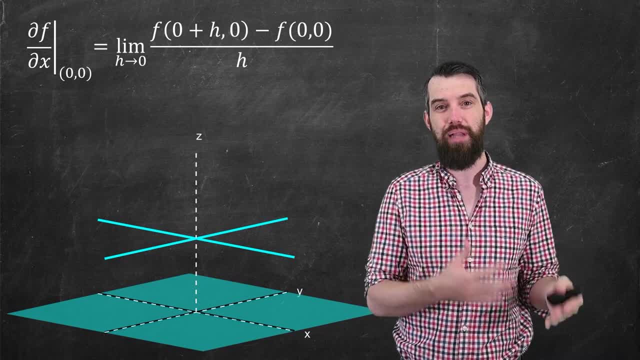 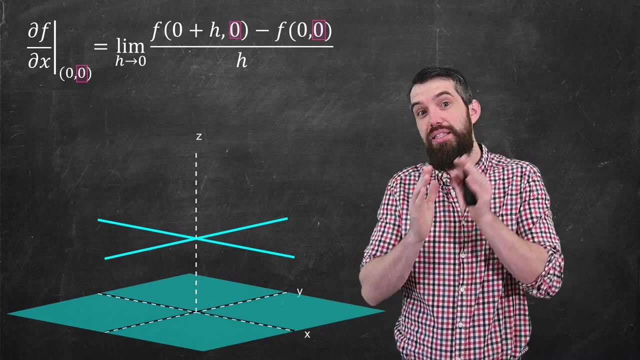 and in this limit the function is evaluated at a couple different places In the y coordinate. well, it's just zeros everywhere. So in other words, the partial with respect to x is thinking of as the y value fixed and only changing the x. 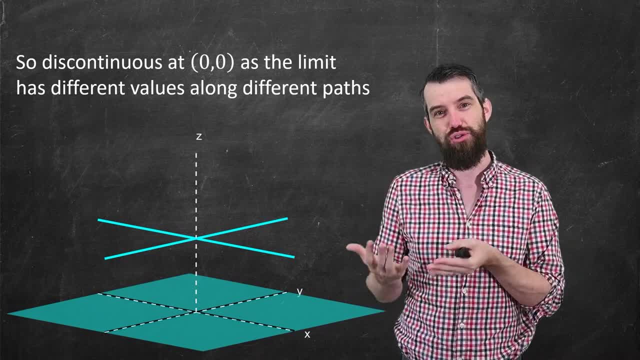 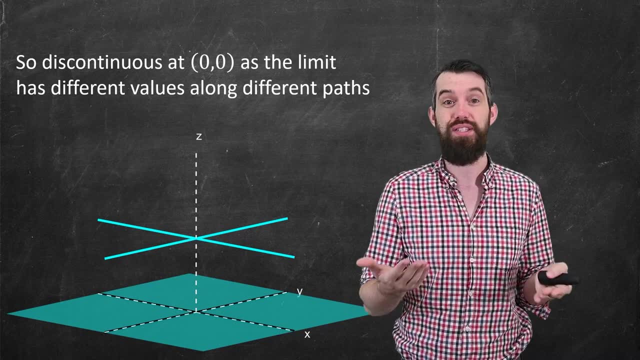 Okay. so if what was true in calculus 1 was true here, we would therefore be able to immediately say: the partial derivatives did not exist. so simple. So let's try to study the partial derivatives and see what happens to them. So let's do the partial derivative with respect to x first. So partial derivative of f with respect. 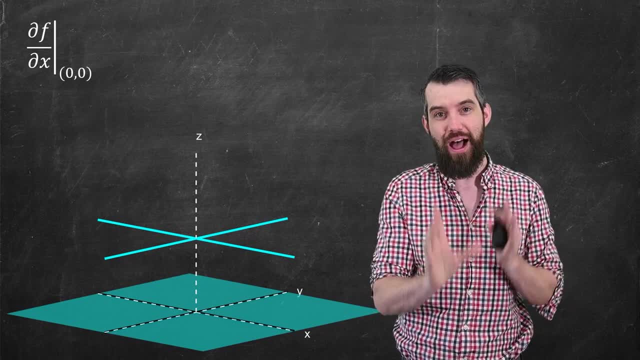 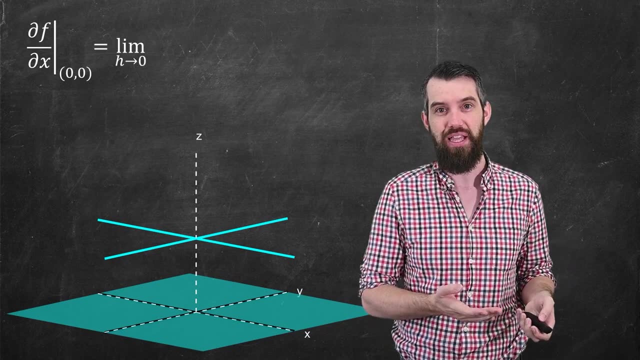 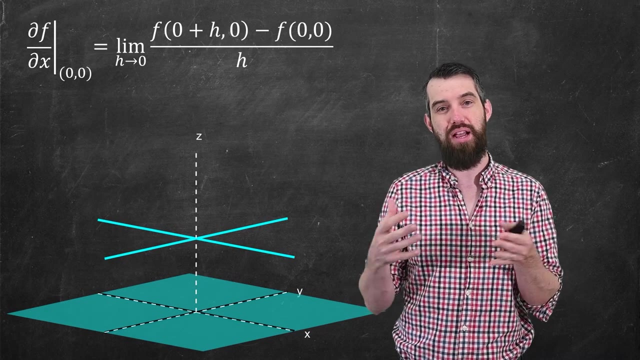 to x and at the point 0, 0.. So that's what the vertical bar means, evaluated at 0, 0.. The definition of partial derivatives, as we've seen previously, is well, it's analogously a limit And in this limit the function is evaluated at a couple different places In the y-coordinate. 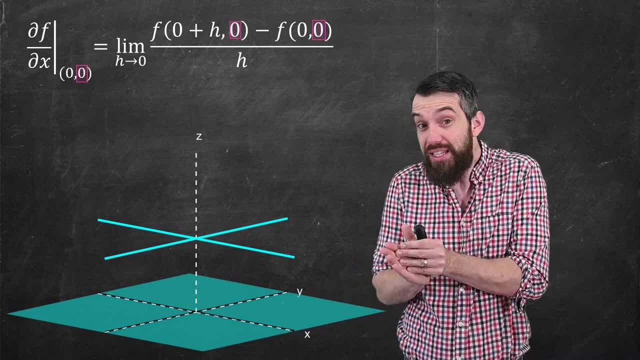 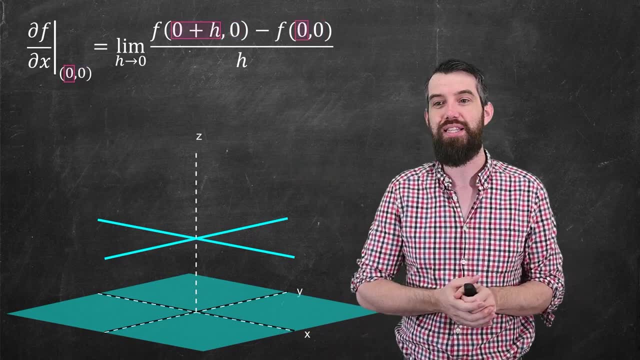 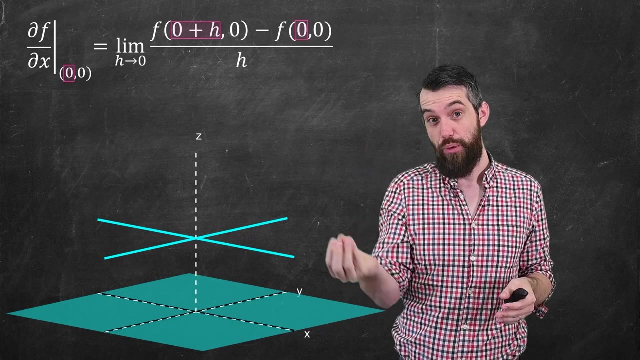 well, it's just 0s everywhere. So, in other words, the partial with respect to x is thinking of as the y value fixed and only changing the x. But then likewise, if you focus instead on the x components, well, the x components change. The one point we're evaluating has an x component of 0,. 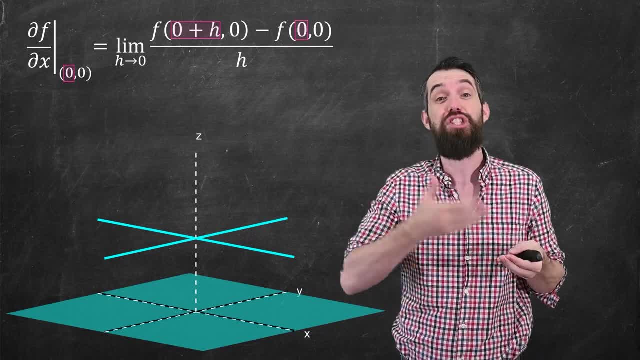 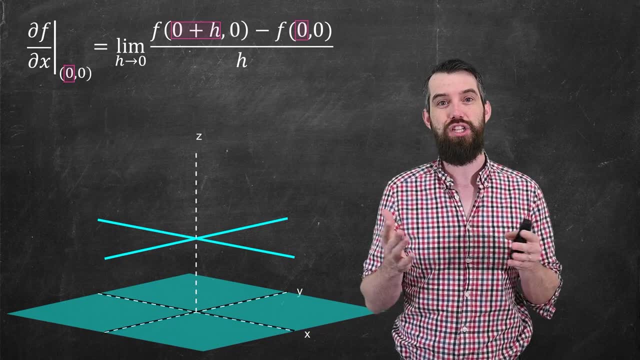 and the other point has an x component of 0 plus h. It's being shifted by this little amount, h that we're taking the limit of and assuming is going to 0.. So this is our definition. Now let's actually try to compute this. 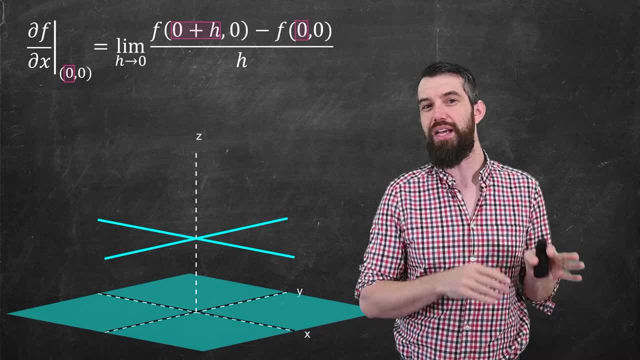 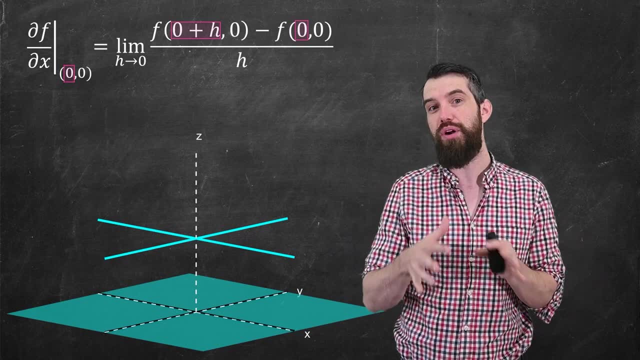 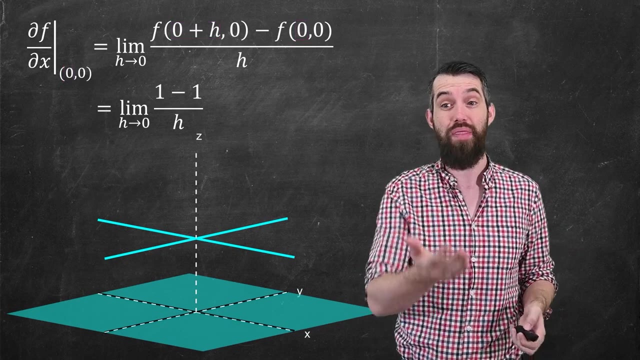 In this case, the x component actually doesn't matter because the y component is 0 in both cases, And this function is a function- that if the y component is 0, then the function has a height of 1.. So both of these expressions on the top are just the values of 1.. 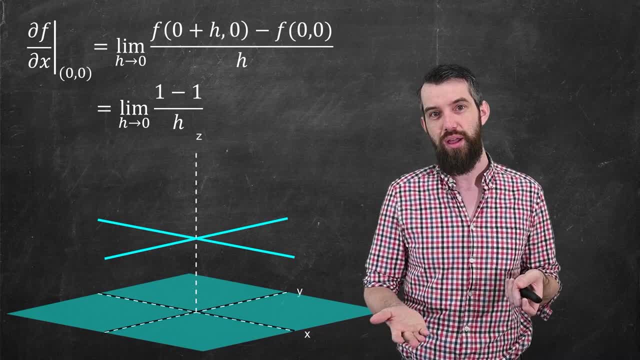 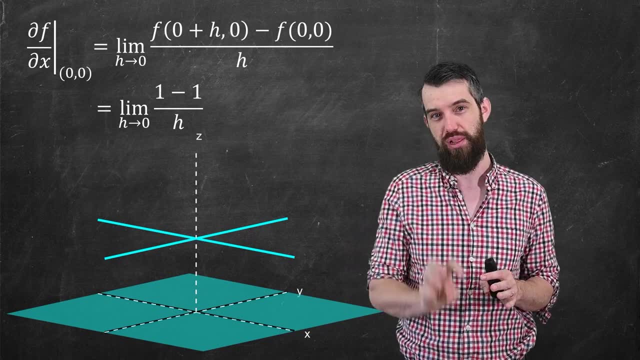 This is just the limit of 1 minus 1.. 1 minus 1 is 0.. It's a little bit weird. You might think this is a 0 over 0, but it's not quite the same. It's a true 0 on the top and then something getting closer and closer to 0.. 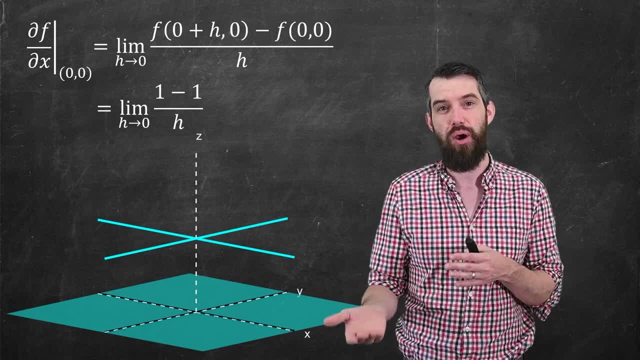 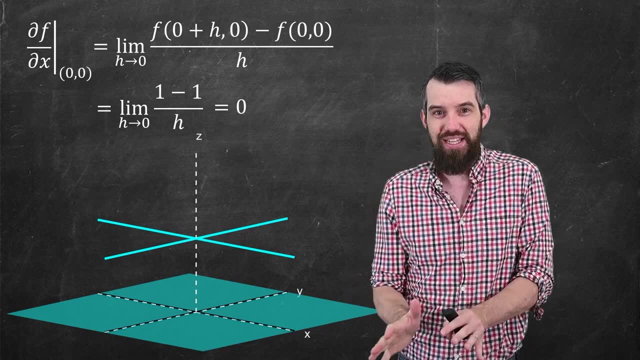 So at any value of h that's non-zero, then we have 0 divided by something. Either way, it's always just going to be equal to 0. So this is surprising. now The partial derivative exists. It's equal to a specific number. 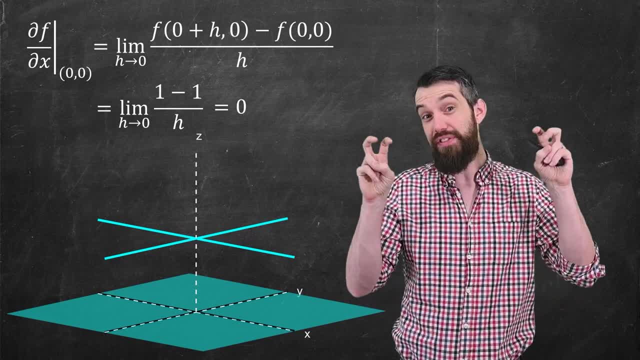 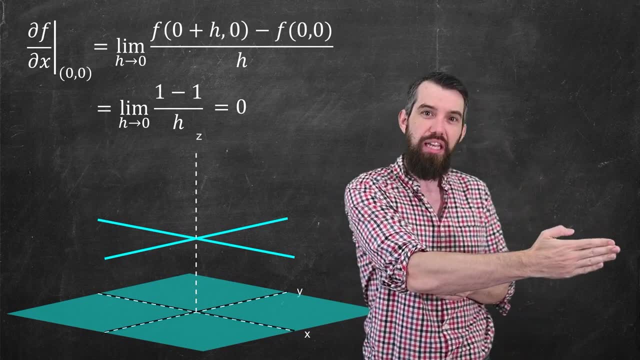 And one of the ways that I think about this is: what does a partial derivative see? Well, it fixes that value of y equal to 0, and then it imagines the x value is changing. It's only looking as you change the x value, It's only looking down the x axis. 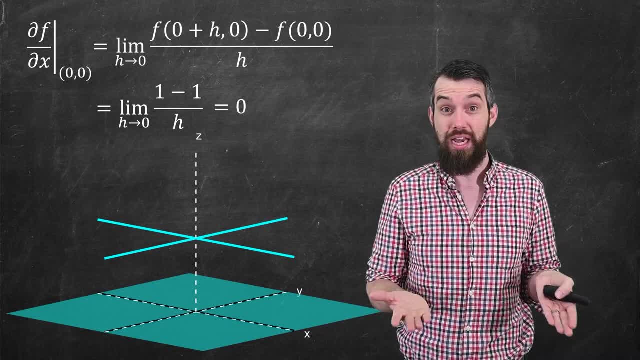 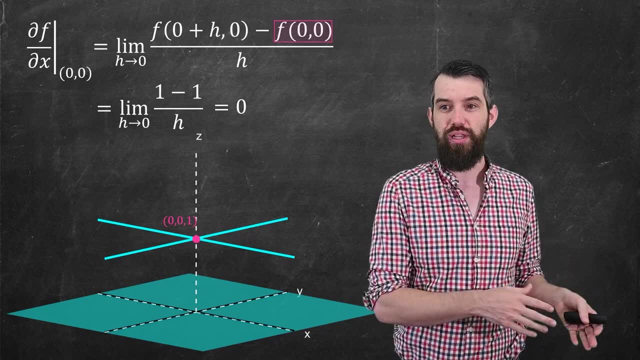 But then the function down the x axis is really nice. It's just a constant 1.. And so the partial derivative from what it can see doesn't see any problems. To look at this a bit more visually, I've plotted the point, which is 0, 0, 1.. 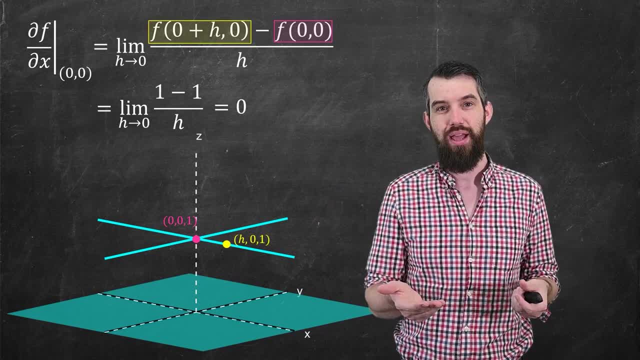 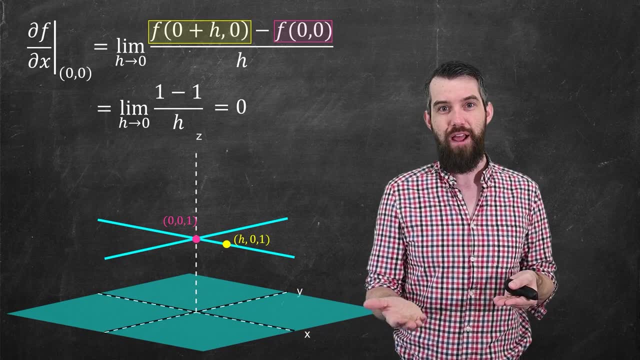 That's what happens. when you plug 0, 0 into f, You get a height of 1.. And then, likewise, if I plug in the point h, 0,, that also has a height of 1.. So those two points I can put them down. And then what do I think of the partial derivative? 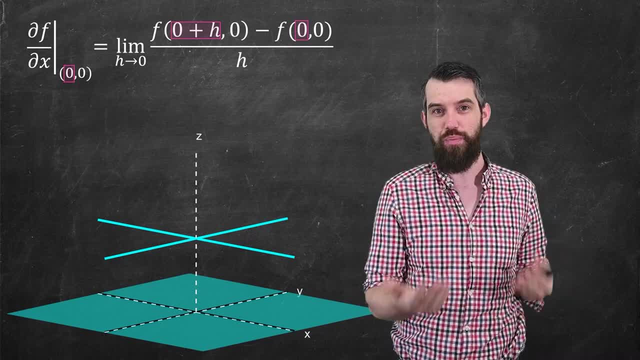 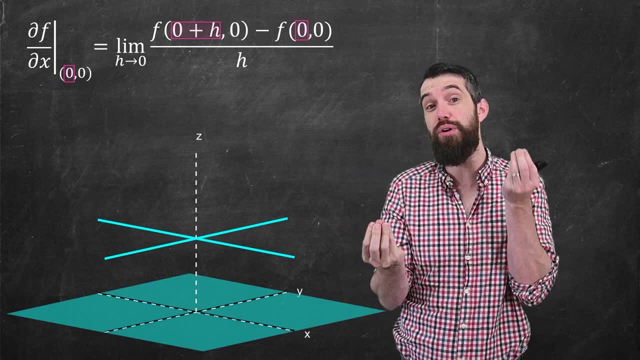 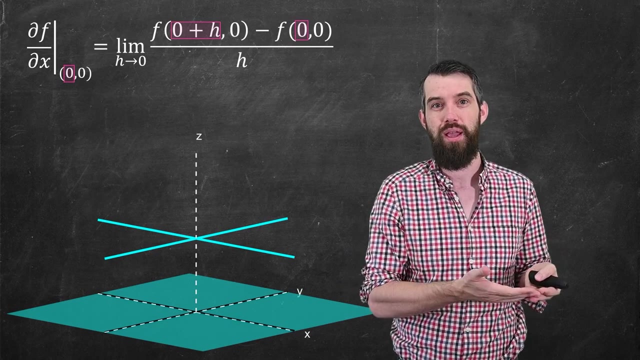 But then, likewise, if you focus instead on the x components, well, the x components change. The one point we're evaluating has an x component of 0, and the other point has an x component of 0 plus h. It's being shifted by this little amount h that we're taking the limit of and assuming is going to 0.. 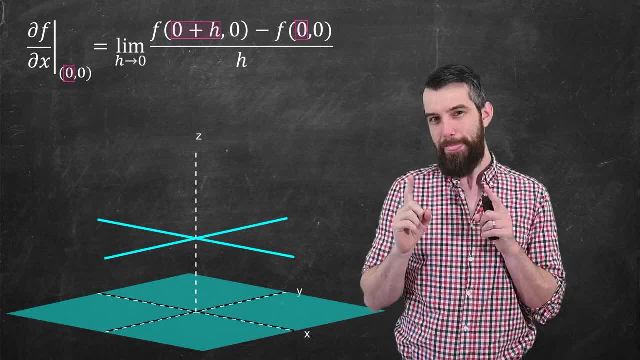 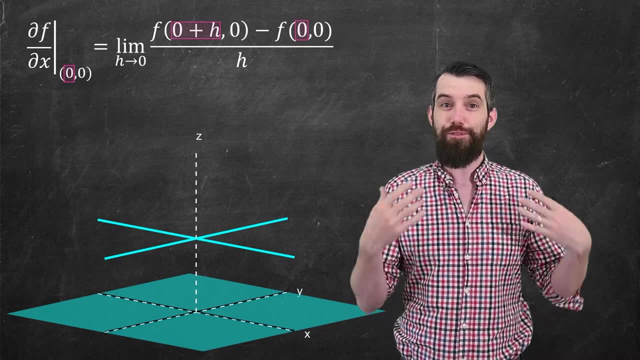 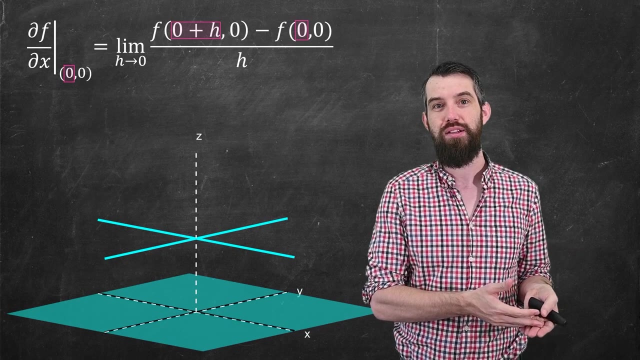 So this is our definition. Now let's actually try to compute this. In this case, the x component actually doesn't matter, because the y component is 0 in both cases And this function is a function that if the y component is 0, then the function has a height of 1.. 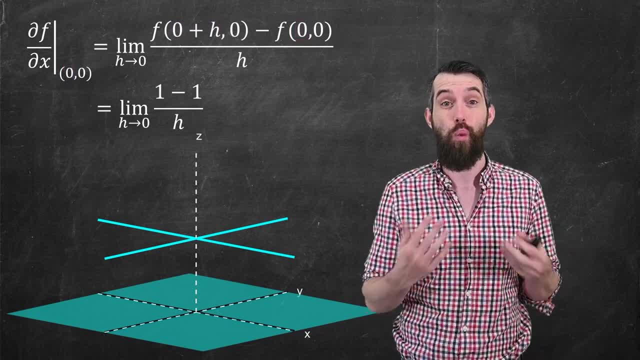 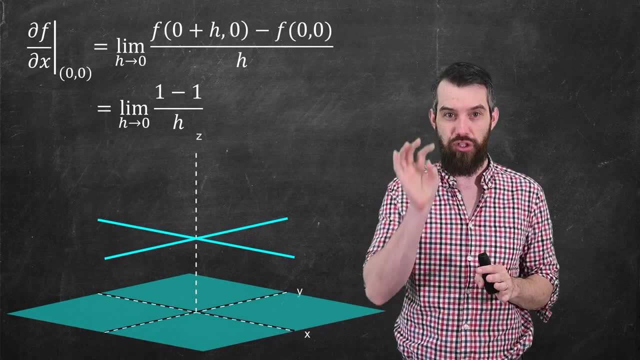 So both of these expressions on the top are just the values of 1.. This is just the limit of 1 minus 1.. 1 minus 1 is 0.. It's a little bit weird. You might think this is a 0 over 0, but it's not quite the same. 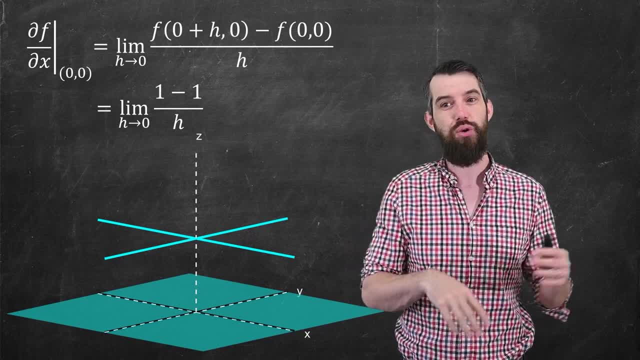 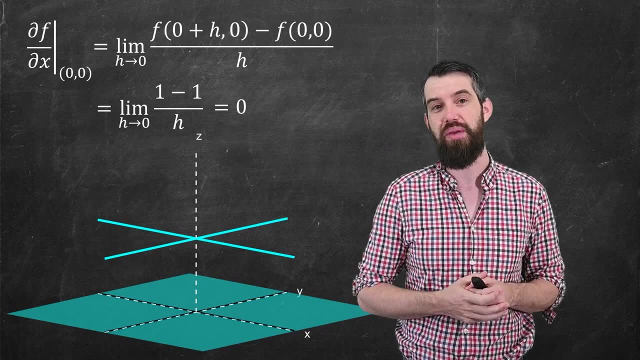 It's a true 0 on the top. It's something getting closer and closer to 0. So with any value of h that's non-zero, then we have 0 divided by something. Either way, it's always just going to be equal to 0.. 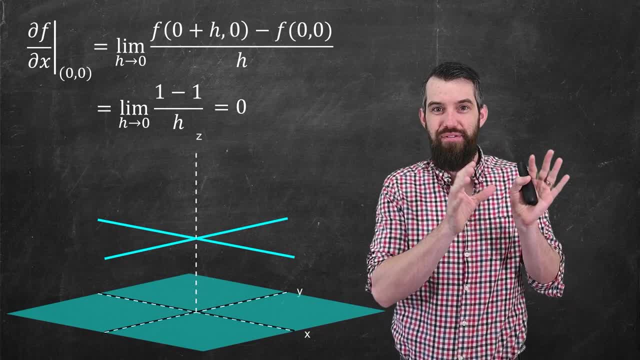 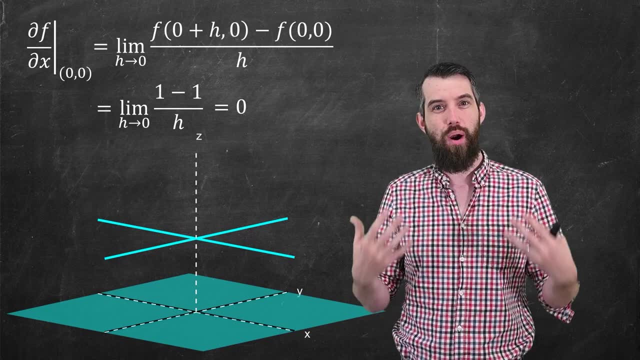 So this is surprising. now The partial derivative exists, It's equal to a specific number, And one of the ways that I think about this is: what does a partial derivative see? Well, it fixes that value of y equal to 0, and then it imagines the x value is changing. 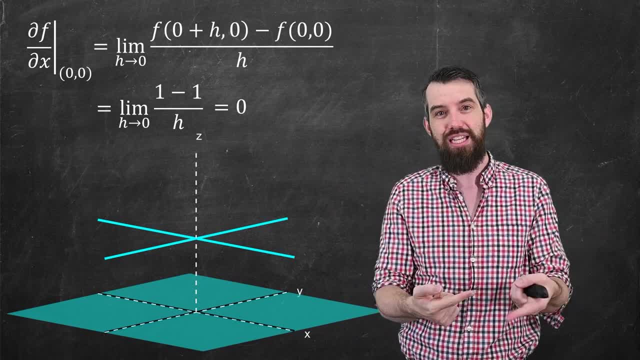 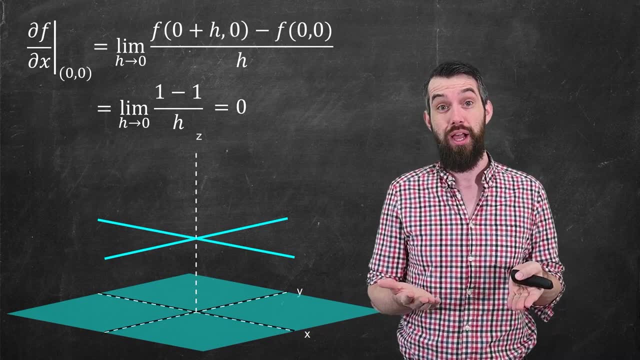 It's only looking. It's only looking as you change the x value. It's only looking down the x-axis. But then the function down the x-axis is really nice. It's just a constant 1. And so the partial derivative from what it can see doesn't see any problems. 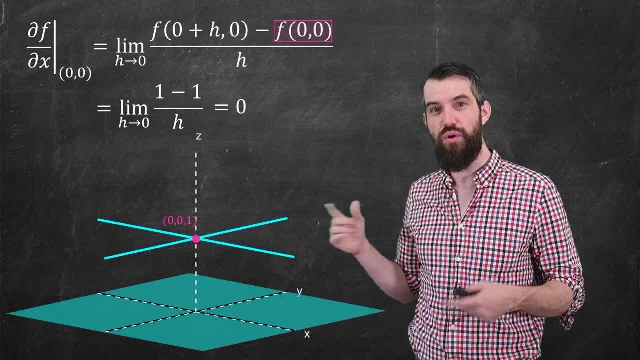 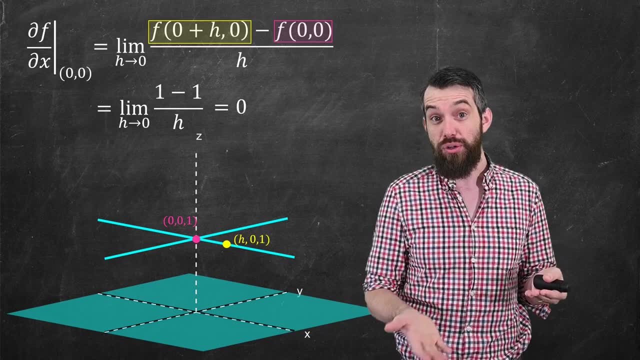 To look at this a bit more visually, I've plotted the point which is 0, 0, 1.. That's what happens when you plug 0, 0 into f: You get a height of 1.. And then, likewise, if I plug in the point h, 0,, that also has a height of 1.. 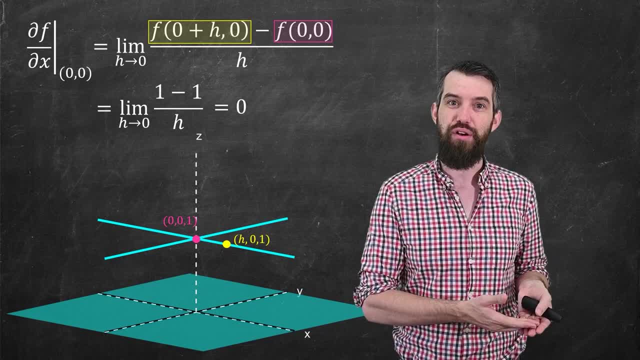 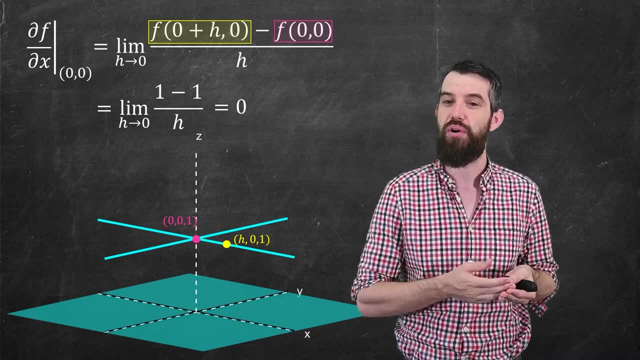 So those two points, I can put them down. And then, what do I think of the partial derivative? The partial derivative is the slope of that secant line between these two points And the limit, as h goes to 0. But because these two points lie on a horizontal line, the slope between them is just 0.